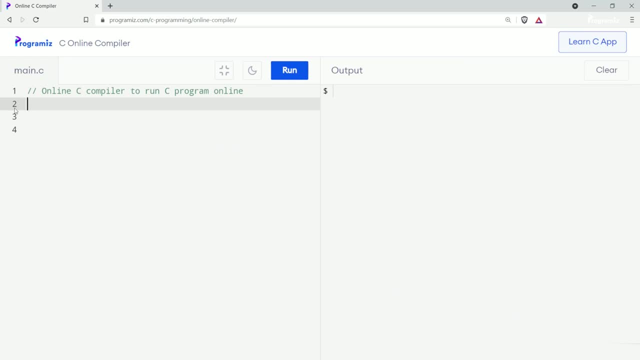 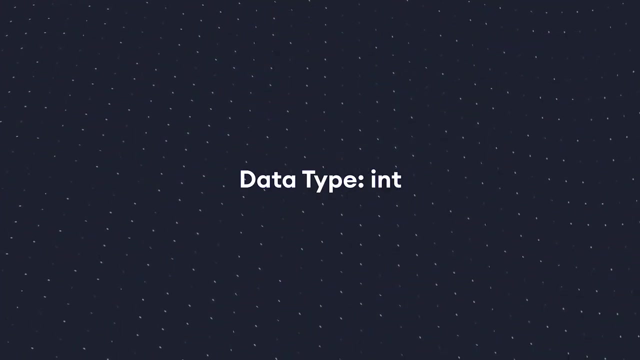 Let me copy a list of data types here in our text editor so that it's bit easier for us to see what they are used for. Now let's try these data types in our program one by one. We have already discussed this. int type variable can only store integer values. 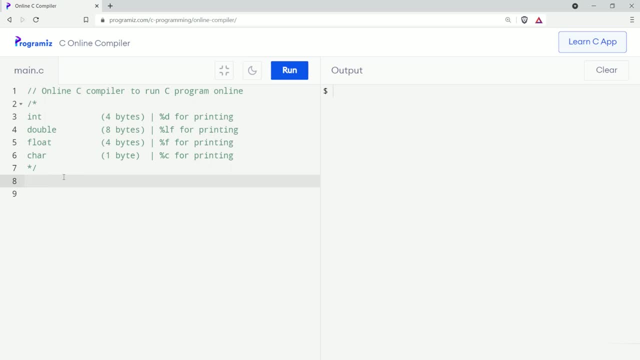 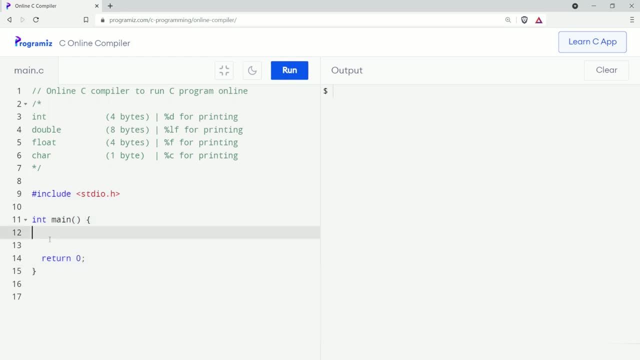 outline of every C program. So I will continue on this And I will assign int as equals to 10.. Here you can see I have assigned 10 to our int variable. as Now, let's print this using printf function: printf, printf, printf. 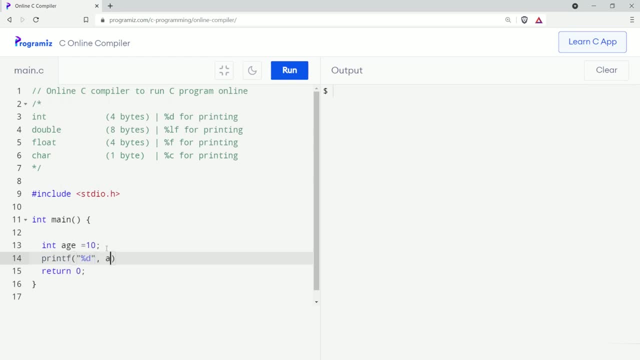 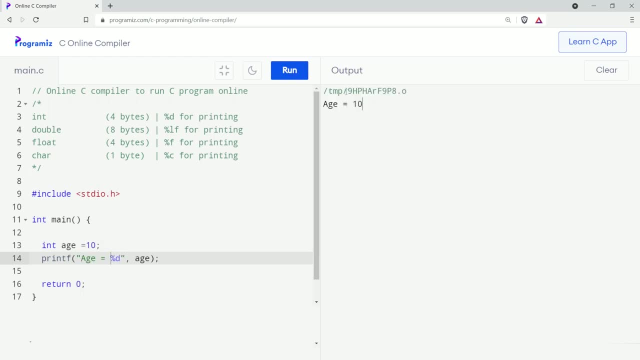 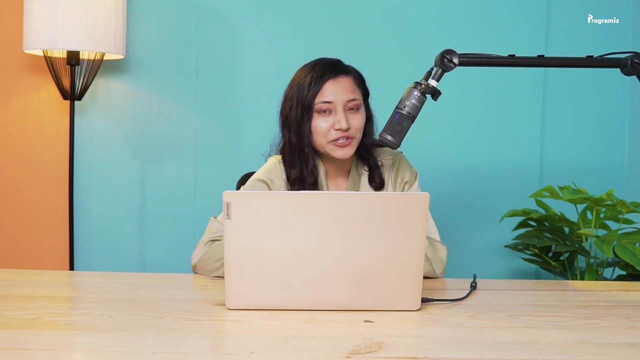 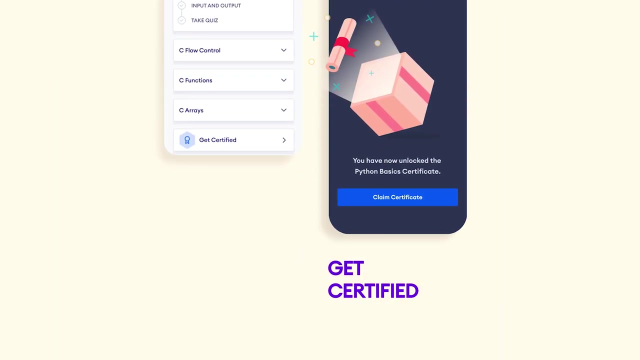 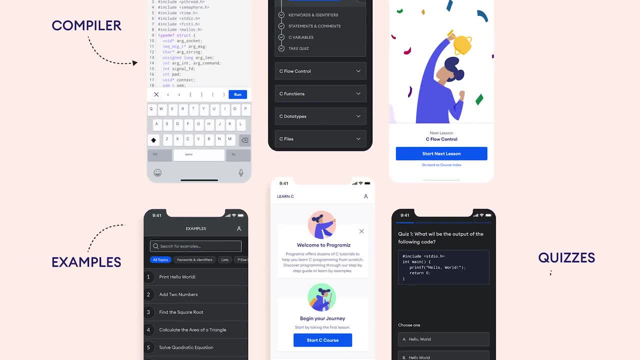 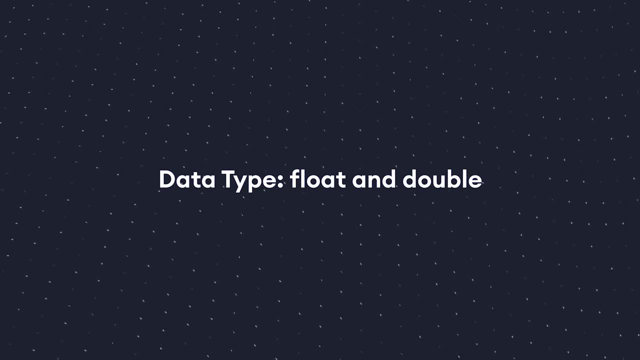 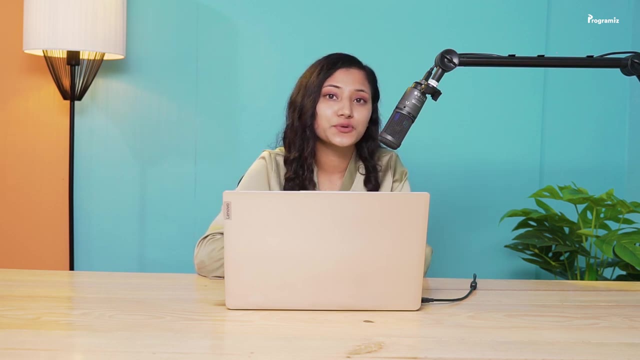 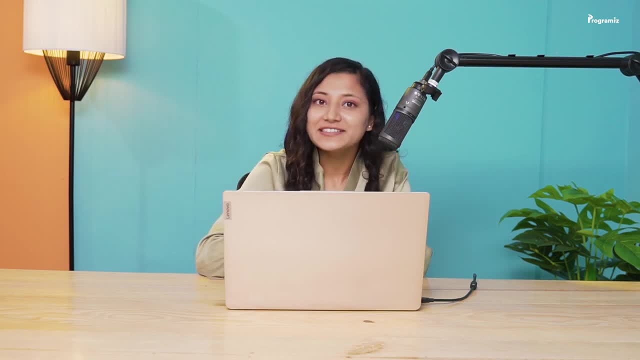 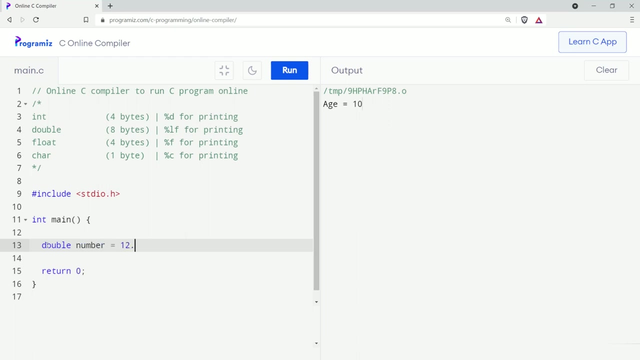 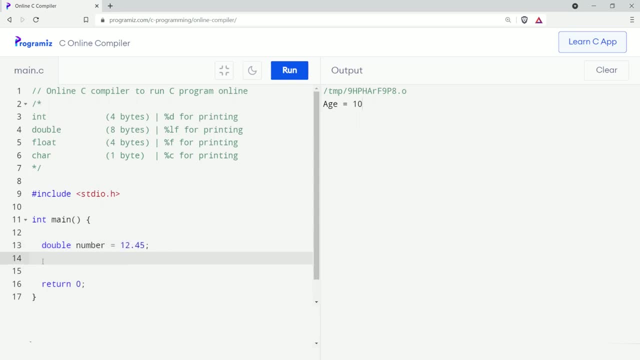 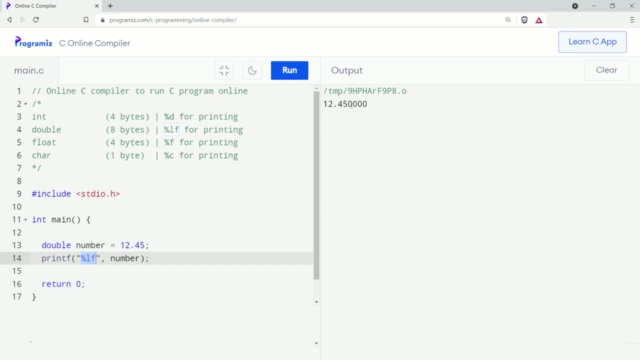 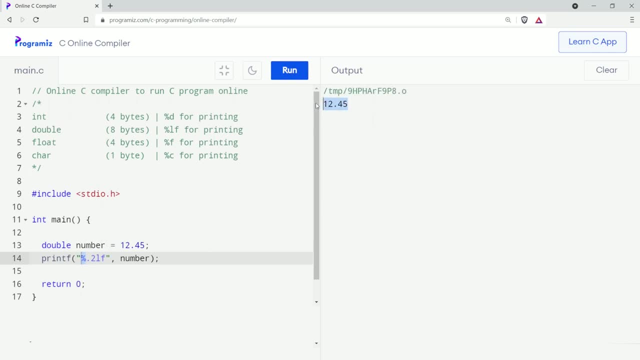 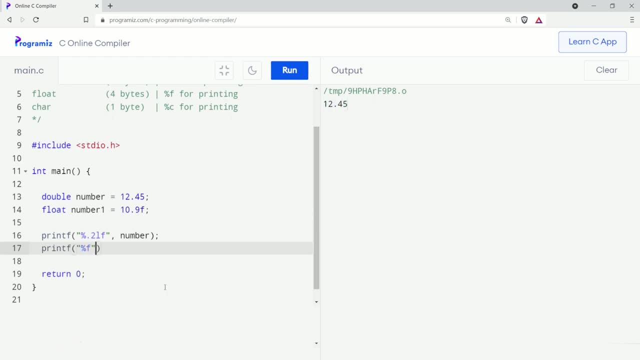 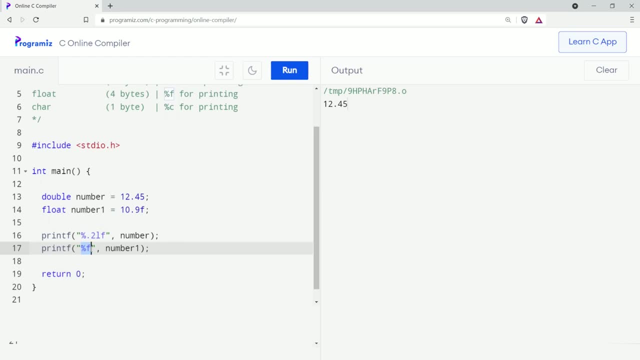 specifier we use for the float variables. Now let me run this code. As you can see, our output is bit messy, so I'll use backslash n here to make our output much more readable. Let's run this again and you can see the output here As in double. we can also remove. 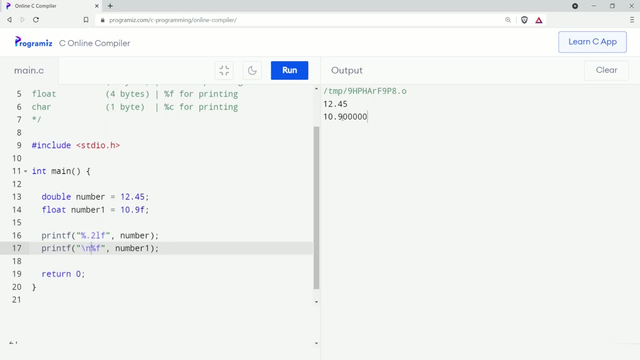 the unwanted digits after the decimal in float as well. Let's try it. I'll add here 0.1 after the percentage and I'll run this And, as you can see, we get the desirable output. By the way, we can also use double and float to store exponential numbers. Let me give. 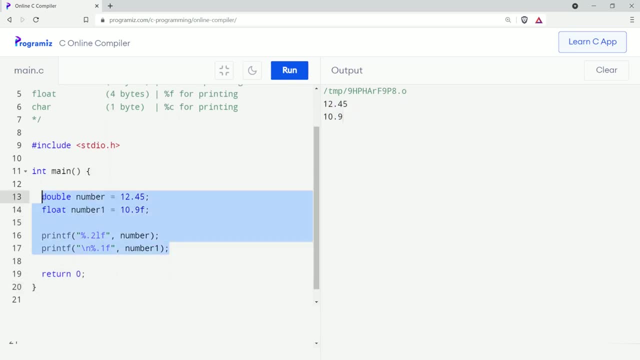 you an example. First I will clean up my editor. Now let me store an exponential number. Double number equals to 5.5 exponential 6.. Here, 5.5 e6 is equals to 5.5 into 10, to the power 6.. Let 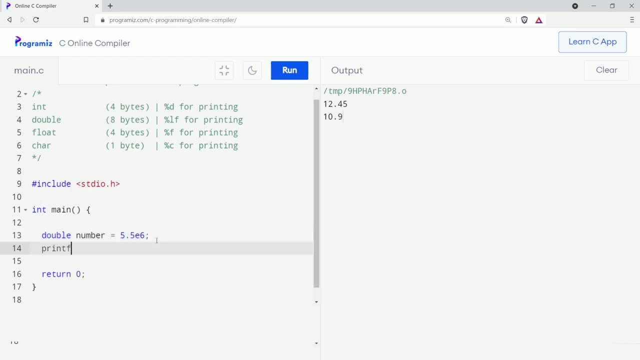 me print this number to verify this. Now let me run this code. As we can see, this number is indeed equals to 5.5 into 10, to the power 6.. Here is a tip for you, Even though both float and double can be used for 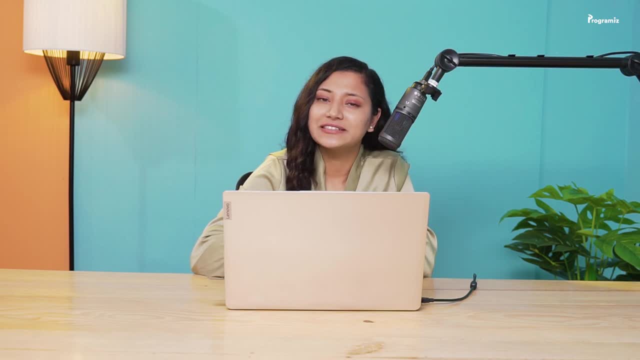 floating point numbers. we suggest you to use double, simply because double can store decimal parts with more precision for larger numbers. Okay, guys, we need your support to keep these types of content on our channel. Thank you for watching. See you in the next video. 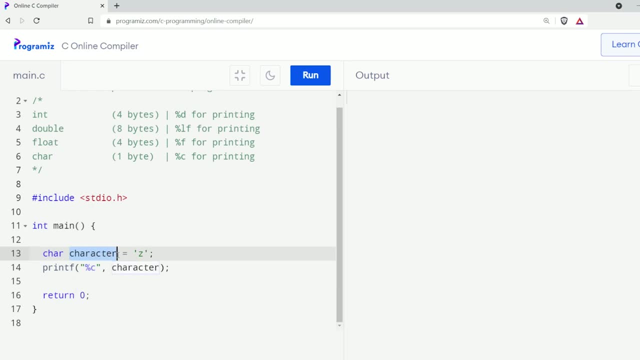 here character is a char variable and i have assigned jet to this character variable. and notice we have used this single quotes for character data. and also notice i have used percent c format specifier for the char variable. when i run the code i'll get the character jet. 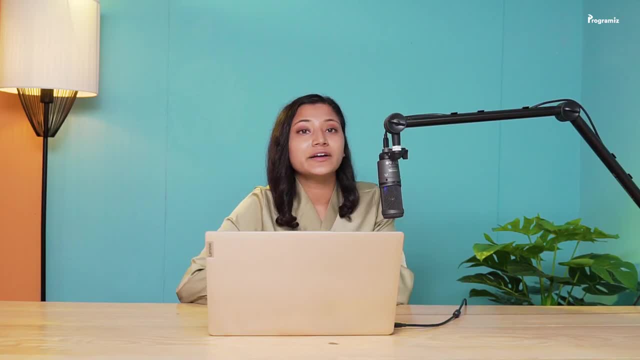 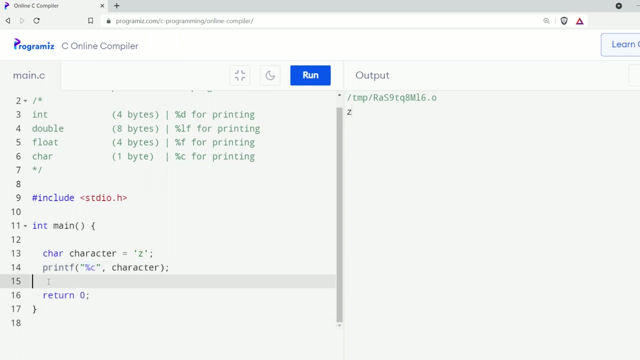 as an output. technically speaking, a character data is internally stored as an integer rather than the character itself. so if we use percent d to print a char variable, we can see its equivalent integer value. so i'll go back to my code editor now. i'll print its integer value. print f bracket.